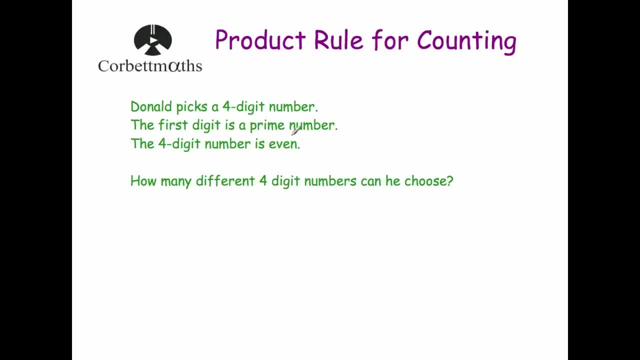 donald picks a four digit number. the first digit is a prime number and the four digit number is even. how many different four digit numbers can he choose? so what we're going to do is we're going to look at each of our four digits again. so we've got the first digit, the second, the third and the fourth. 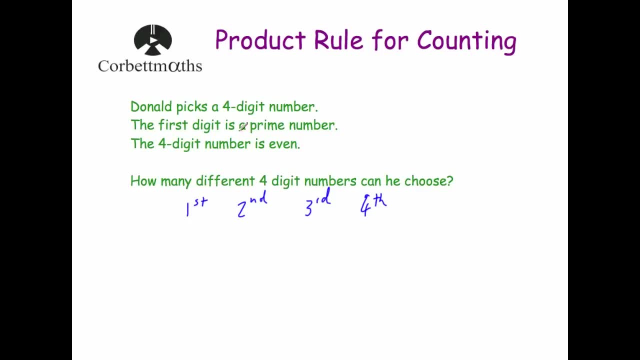 okay now, first of all, it says the first digit is even, or sorry, the first digit is a prime number. okay, so the first digit is a prime number. so the prime numbers are: well, the prime numbers are two, three, five, seven, eleven and so on. so there's four different prime numbers. that could be the first digit, and so we're going to put four. 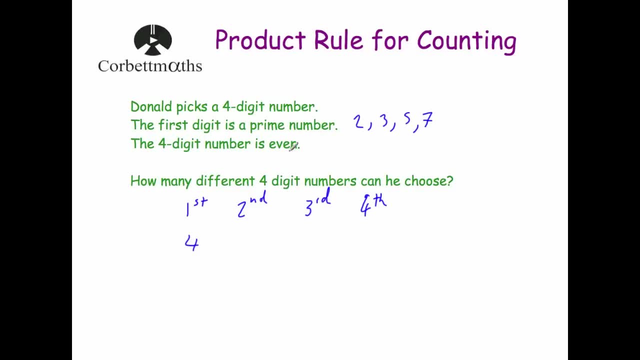 there. next it says the four digit number is even. now. that only affects the last number. okay, the last digit, because obviously, to be even, it's going to end in a zero: two, four, six and eight. so there's five different numbers, which would you know? one of these five has to go on the. 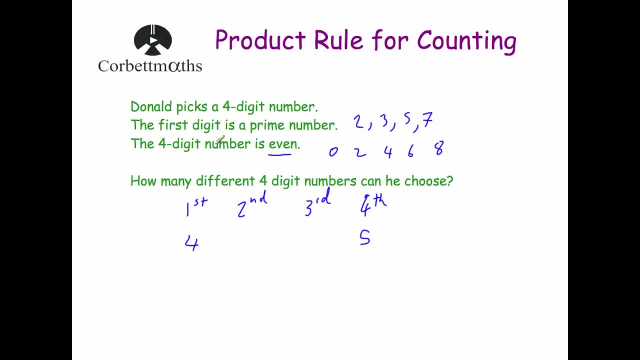 end of the number. to make it even so, it means there's a five there. now the second digit and the third digit of the number. well, we don't actually have anything else. that sort of you know restricts what they can be. so that means there's ten. 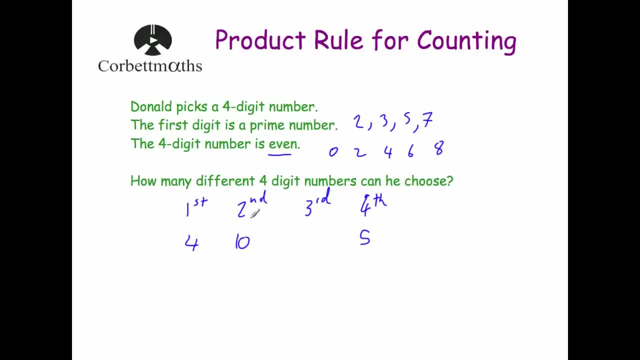 different options for the second digit, that's zero, one, two, three, four, five, six, seven, eight, nine, and likewise for the third digit. so what we're going to do is we're just going to multiply these together, and then that will tell us how many different possible four digit numbers you can. 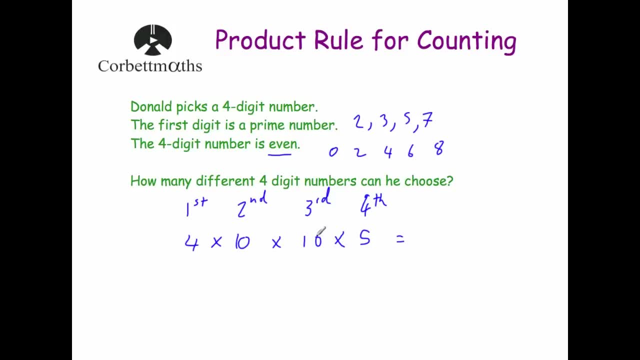 choose. so four times ten, forty times by ten, four hundred times by five, two thousand. so there's two thousand different possible numbers that donald could have been thinking of. okay, our second example. kitty has 52 different playing cards. she gives one card to grace, she then gives one card to bill and she gives one card to jenny. and how many different ways can kitty do? 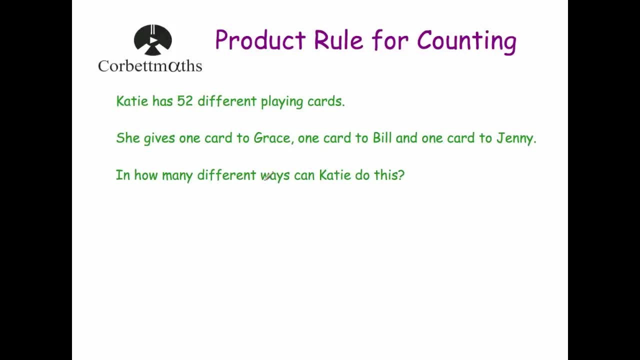 this. now, this question is slightly different than the other ones, and you're going to see why now. okay, so first of all, we're going to give a card to grace, a card to bill and a card to jenny. now, first of all, she's going to give a card to grace. now, there's 52 different cards. she can give any. 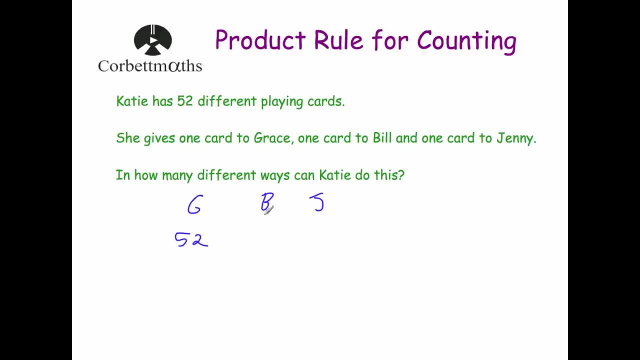 of those to grace. so there's going to be 52 there. now for bill, she's going to give a card to jenny. she's going to give him one card to grace. so that means there's 51 possible options that she could give the bill, because obviously if she's given one away, there's only 51 cards left in the. 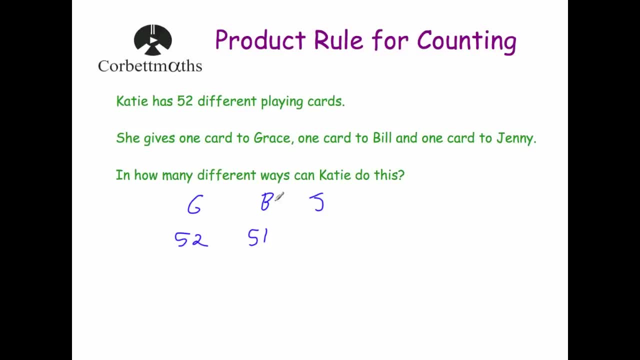 deck. and then for jenny: well, if she's given a card to bill now, that means there's only 50 cards in the deck. so that means that in how many different ways can katie do this? we would times 52 by 51, by 50 and 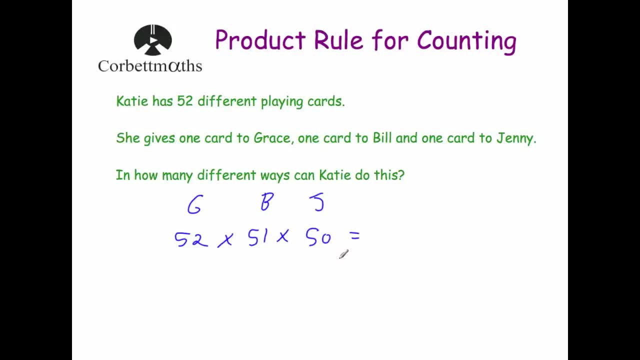 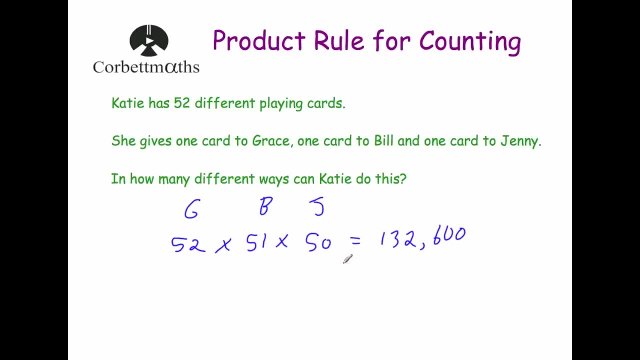 if we multiply those numbers together, that will tell us what our answer is. what we do is calculation is: So there's 132,600 different ways that Kayleigh can give one card to Grace, one card to Bill and one card to Jenny. Okay, our next question. 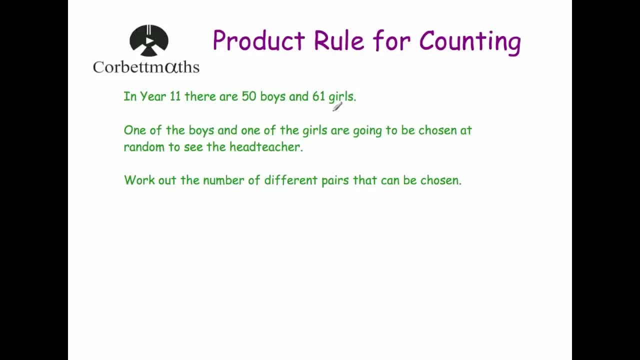 So the next question says: in year 11, there are 50 boys and 61 girls. One of the boys and one of the girls are going to be chosen at random. to see the headteacher Work out the number of different possible pairs that can be chosen. 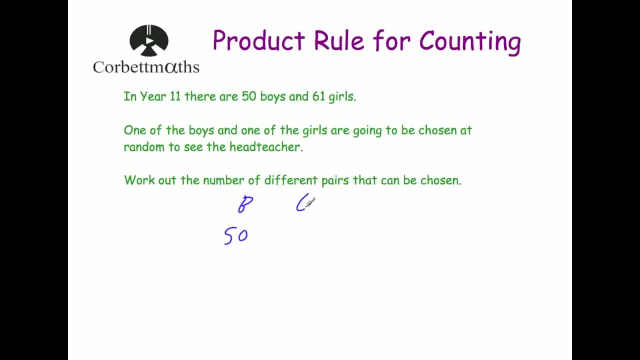 So again, for the boys, there's 50 different boys to choose from, and for the girls, there's 61 different girls to choose from. So to work out the different number of pairs that can be chosen, we just multiply these together. 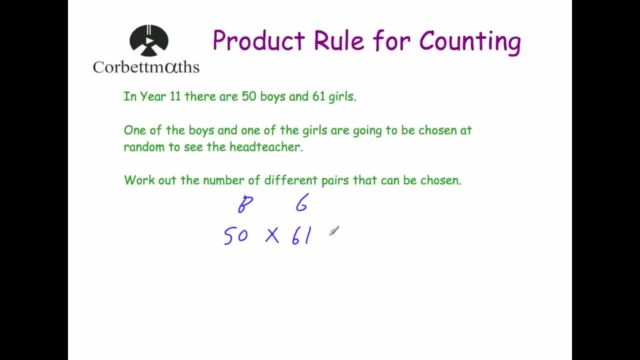 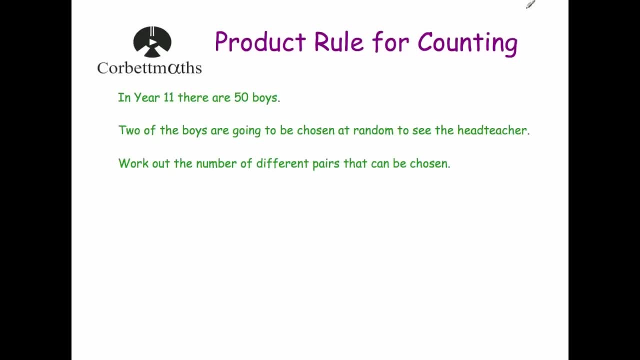 So we just do 50 times by 61, and that gives us 3,050.. So there's 3,050 different possible pairings that we could have. Now. following on from that, our next example says: in year 11, there are 50 boys. 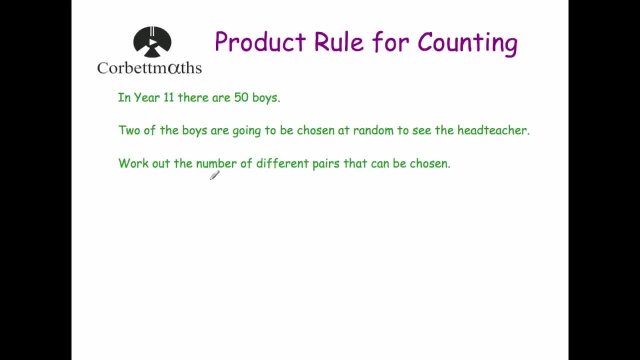 Two of the boys are going to be chosen at random to see the headteacher Work out the number of different pairs that can be chosen. So this time we're going to have a look at the first boy and the second boy. Now, first of all, we've got 50 boys to choose from initially. 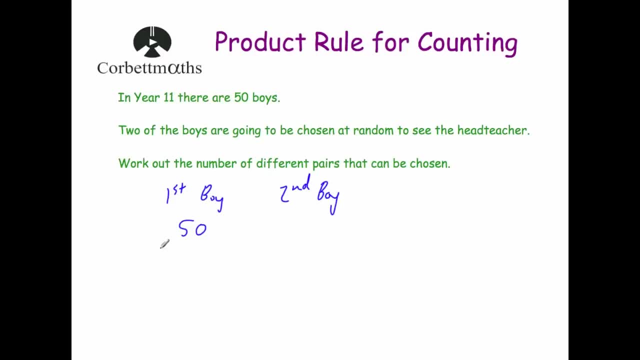 So for the first boy selected, there's going to be 50 different boys that can be chosen from, And that means that if one of those is chosen, that only leaves 49 for the second one. Now we're going to times those two together. 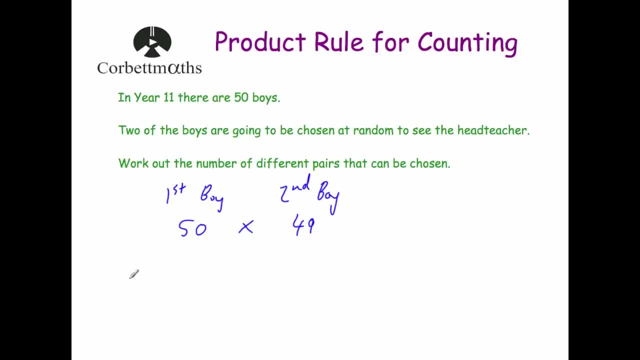 Now, before we sort of think that's just a final answer, we need to consider this. For instance, if I had two students, just call them Alan and Bob, For the first boy we could get Alan, and for the second boy we could get Bob. 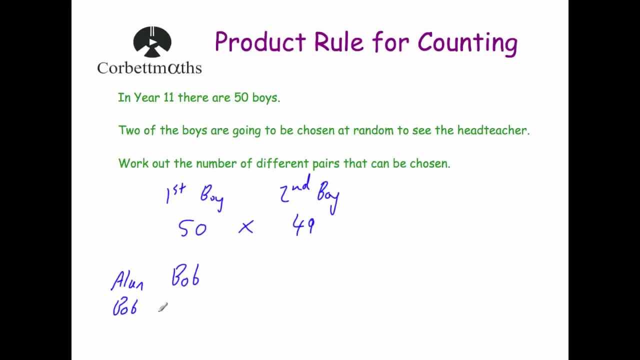 But likewise we could potentially get Bob And then Alan. Now it says: work out the number of different pairs that can be chosen. Now, obviously we don't want to sort of count Alan and Bob as a different pair to Bob and Alan. 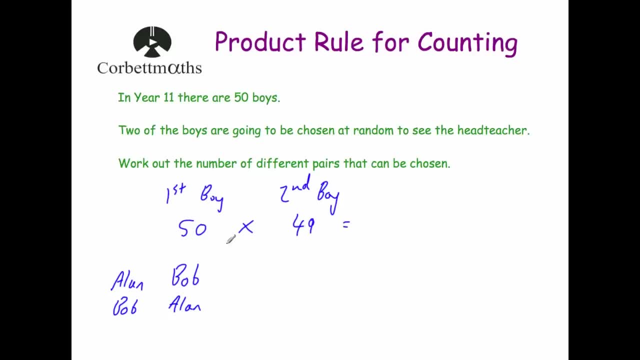 because it is the same pair of students. So what we're going to do is we're going to times these two together and then half it. Now, the reason we didn't do that in the last example is it said: you know, there was 50 boys and 61 girls. 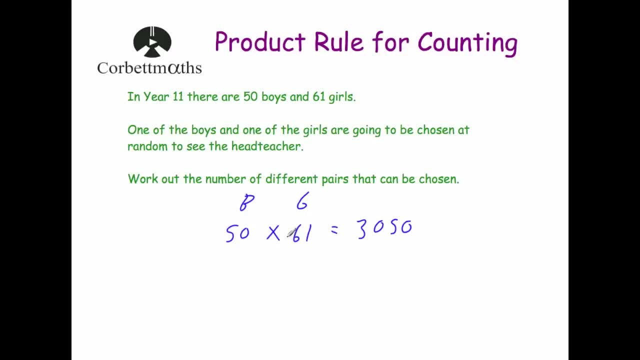 Now, obviously you can't get the boy and the girl. you know the other way, you know mixed up. You know, for instance, if you had Alan and if you had Hannah, you know, if you're picking the boy and then the girl, you can only get Alan and Hannah. 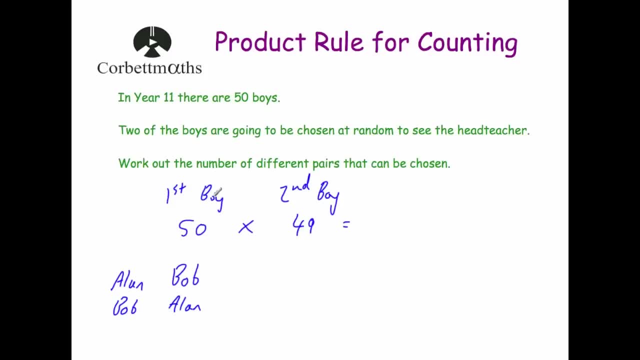 So we don't need to, you know, to half that one, But here because it's boy and then boy and we want to find out how many different possible pairs there can be. you know, we don't want to duplicate the pairs. 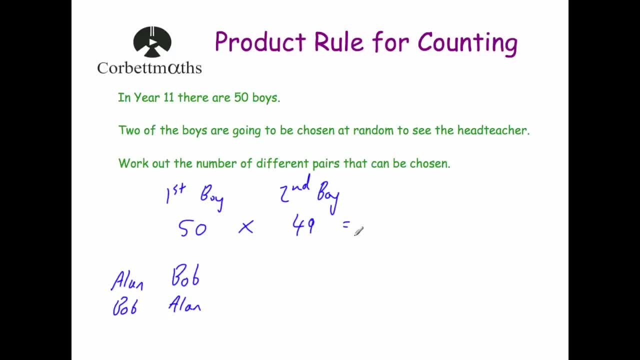 So what we're going to do is we're going to times these together 50 times 49. So 50 times 49 is 2,450.. But then we're going to divide that number by two. And that means that whenever we divide that by two, obviously you know here, you know this: 2,450,. 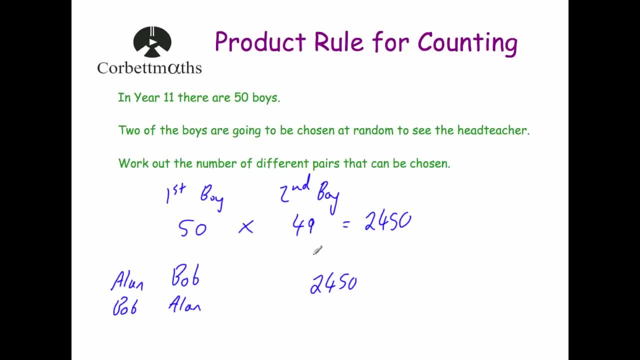 it includes all the possible combinations for the first boy chosen, second boy chosen, But obviously that includes all the duplicates. So we divide it by two and we get an answer of 1,225 possible pairings of students. OK, now last example. 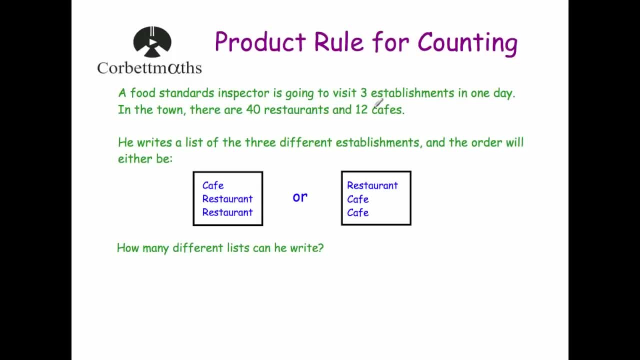 Our last example said a food standards inspector is going to visit three establishments in one day. In a town there's 40 restaurants and 12 cafes. He's going to write a list of three different establishments that he's going to visit And the order will either be: 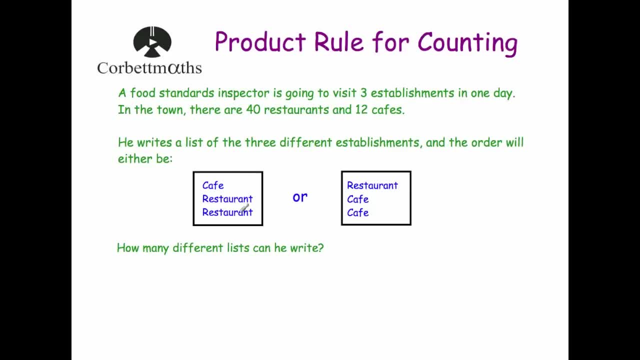 So this particularly is going to do it in and see if we're going to be cafe restaurant restaurant or restaurant cafe cafe. How many different possible lists can he write? OK, so let's first of all look at cafe restaurant restaurant. 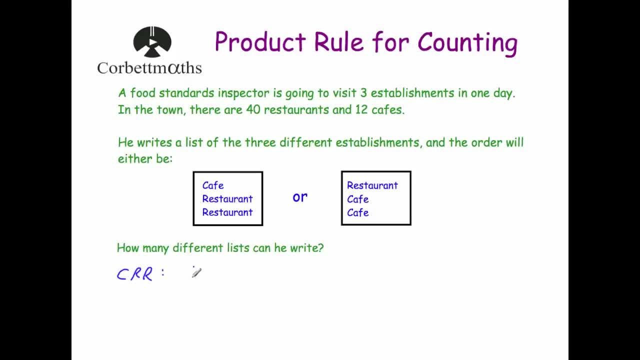 So that's going to be well. cafe to begin with. Well, we've got 12 of those. and then we times that by restaurant: Well, there's 40 restaurants. But given that he's going to visit three different establishments, for the next restaurant he's only going to times by 39.